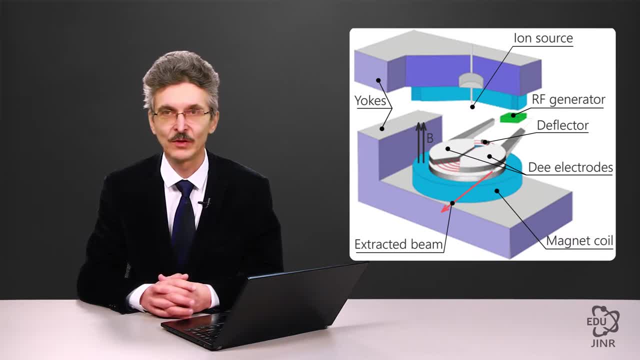 At the center of the magnet there is the ion source. The ions, through their interaction with the electric field of the duons, increase in energy. The orbit radius rises. The orbit looks like a spiral, turning from the accelerator center to its periphery. 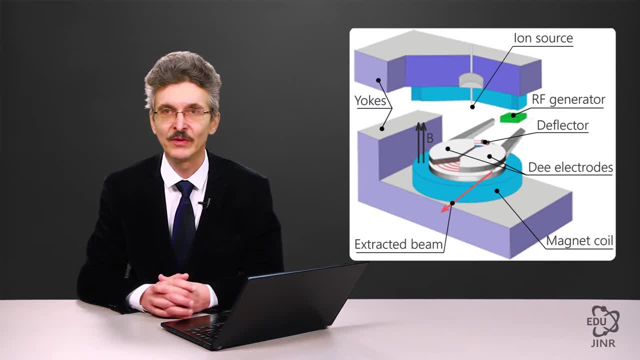 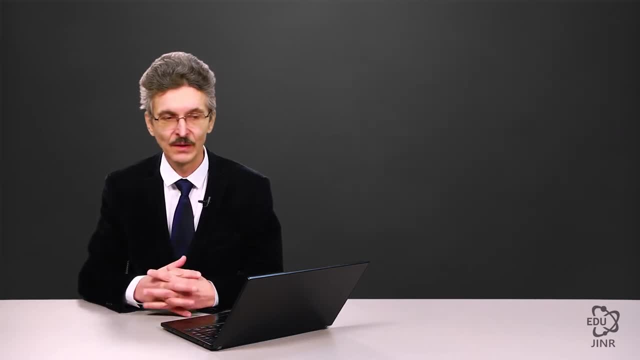 When the particles reach the magnet borders, they get extracted from the accelerator with the use of a special deflector and then utilized for further experiments. It was the cyclotron that was used as one of the first facilities at our institute, Under the guidance of Georgi Fleurov, at the future Fleurov Laboratory of Nuclear Reactions. 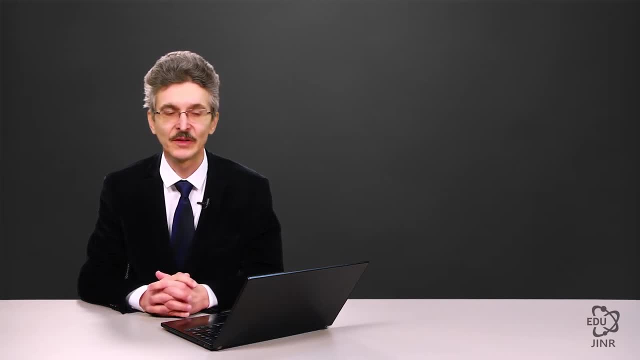 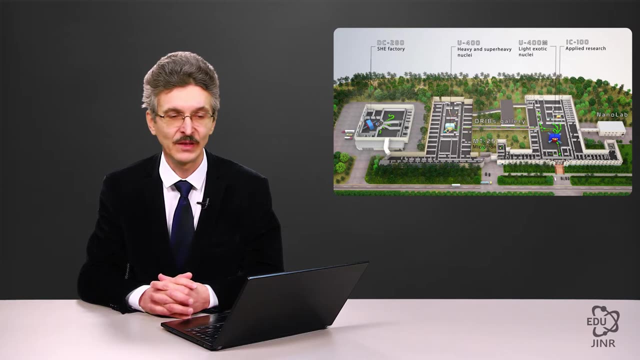 the first specialized heavy-ion cyclotron was created. Today, the construction of a new cyclotron complex is being finalized. The complex will consist of four cyclotrons: A specialized cyclotron for the synthesis of super-heavy elements. a cyclotron for the study of heavy and super-heavy nuclei. 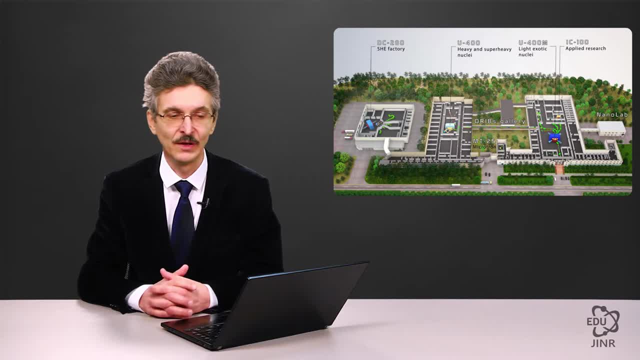 a cyclotron for the study of light exotic nuclei and another cyclotron for applied research. Besides that, the complex will include a laboratory for the research in nano-objects obtained with the help of heavy particle beams, The Fleurov Laboratory of Nuclear Reactions and its program. 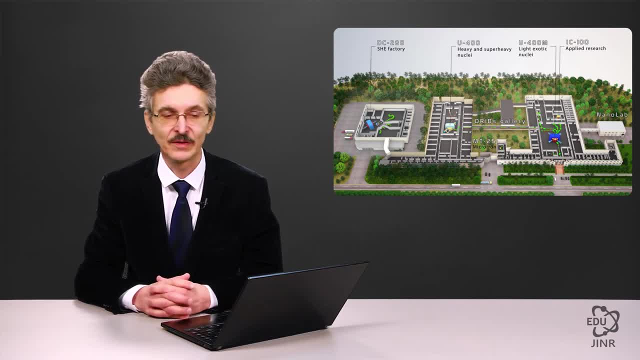 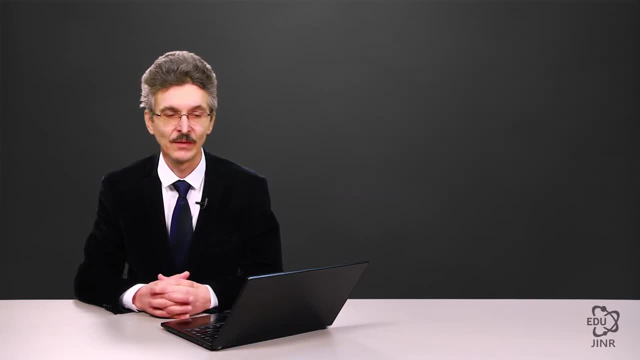 on the heavy-ion cyclotron development have to a great extent determined the international authority of our institute. Currently, the International Committee has prioritized the discovery of numerous new elements for Mendeleev's periodic table. The first among them was named Dubnium. 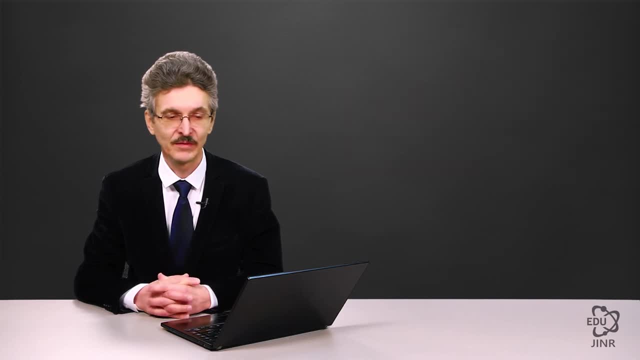 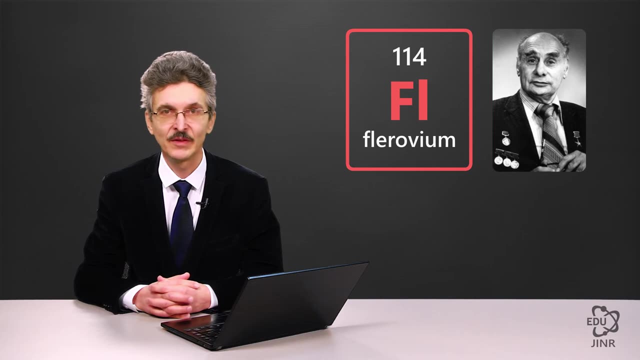 It's the 105th element. Most recently, new names have been given to two other elements. The 114th element has been named Fleurovium, in honor of the founder of the lab, a member of the USSR Academy of Sciences, Georgi Fleurov. 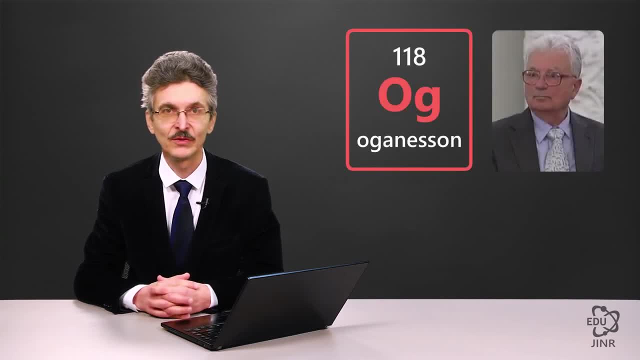 and the 118th element has been named after the lab's current scientific leader, Yuri Oganesyan.